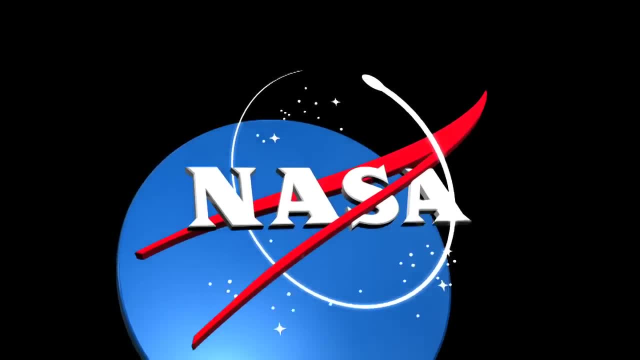 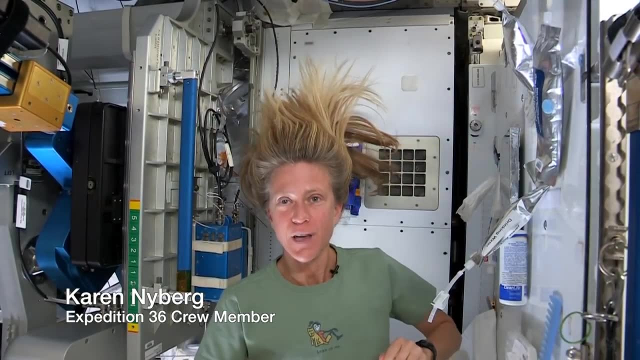 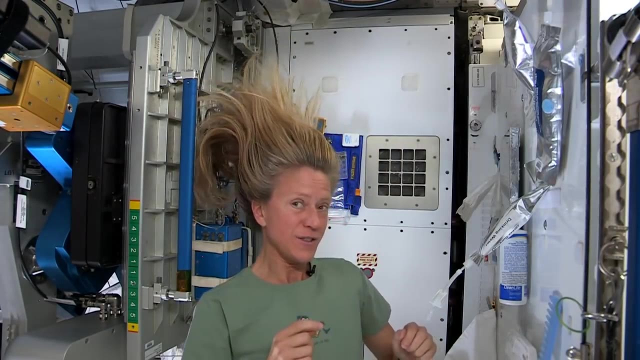 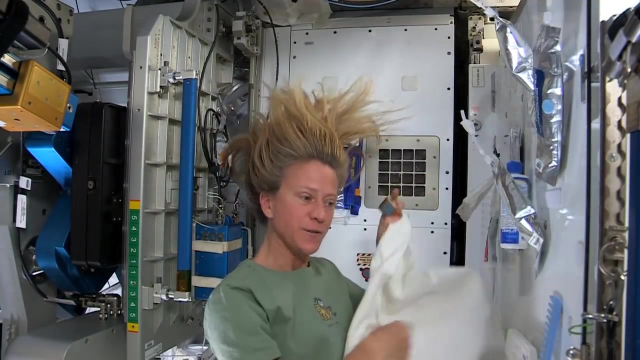 Hi there. I've had a lot of people ask me how I wash my hair in space and I thought I'd show you how I do it. Let's see To get started, these are the things I need: A bag of warm water, a little no-rinse shampoo, towel and my comb. What I like to do is start. 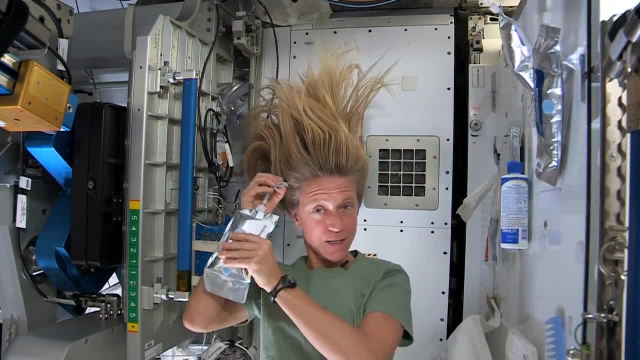 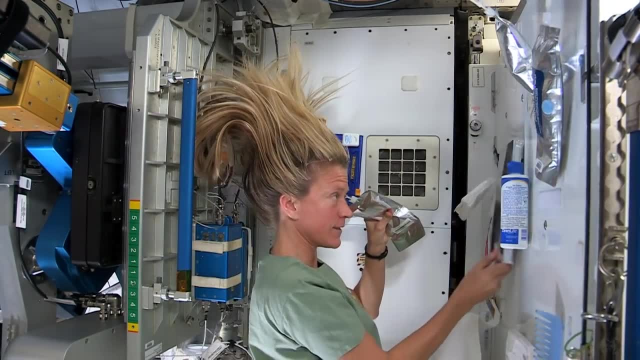 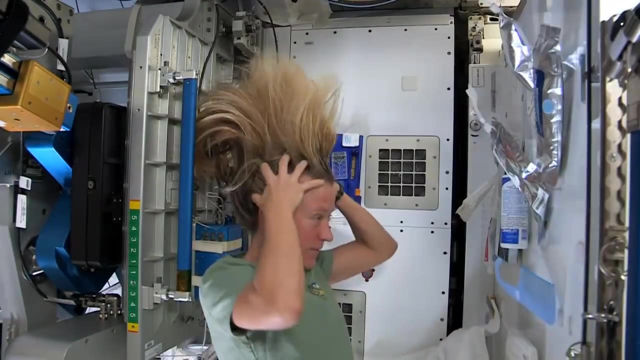 by just putting some hot water, squirting it onto my scalp, And I have a mirror here so I can kind of watch what I'm doing. Sometimes the water gets away from you and you try and catch as much as you can. Then I just work the water up through to the ends of my 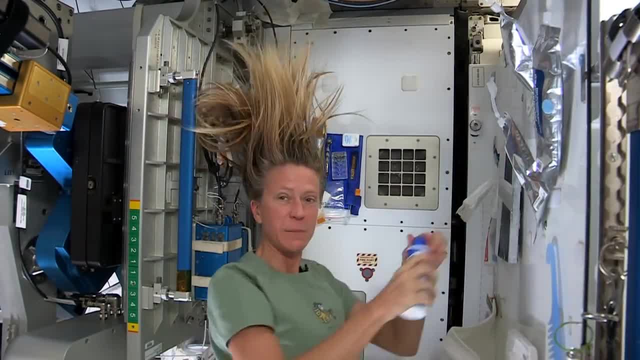 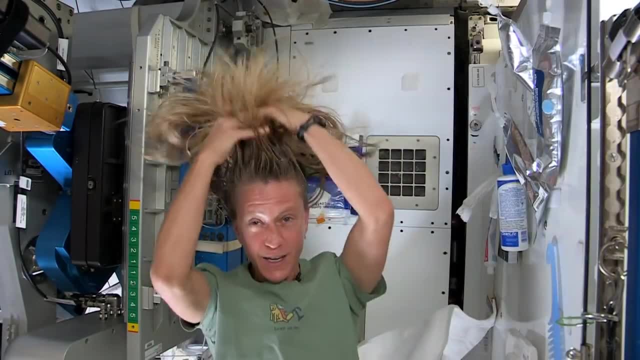 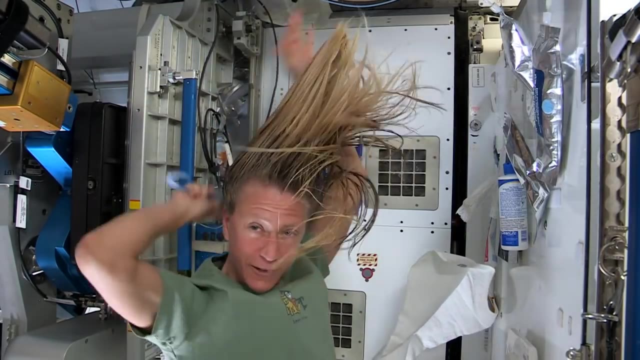 hair. Then I take my no-rinse shampoo and squirt it also on the scalp Just a little bit And rub it in Again, kind of working it out to the ends. And sometimes I'll actually take my comb to help work it all the way to the ends. And I like to take 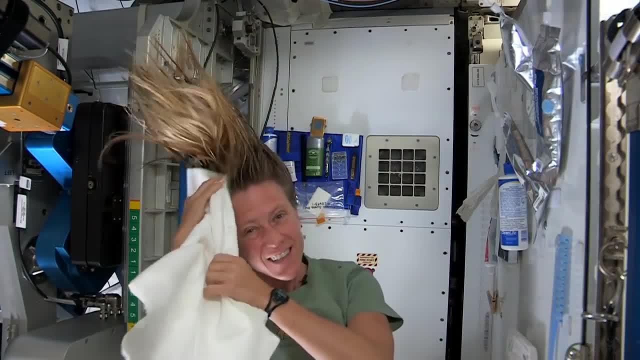 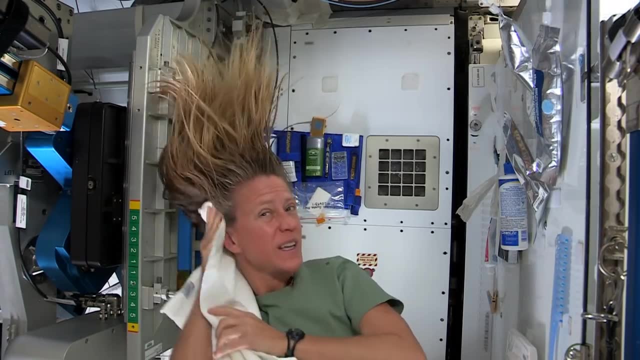 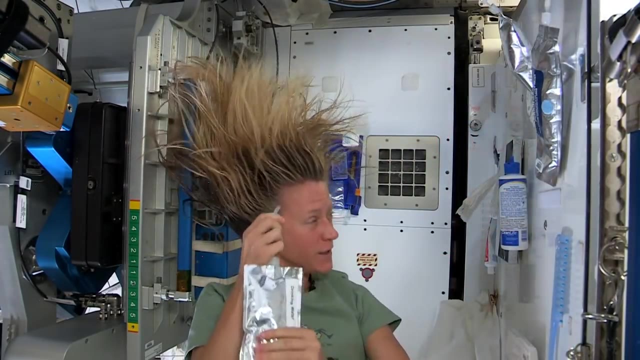 my towel while I have the shampoo in there and just kind of work it, Because without standing under running water, you kind of need to use the towel a little bit to help get some of the dirt out. Try a little more water. It's called no-rinse shampoo, but I think it's best to use a little. 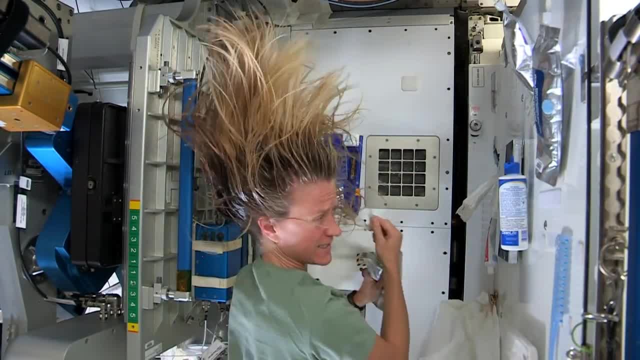 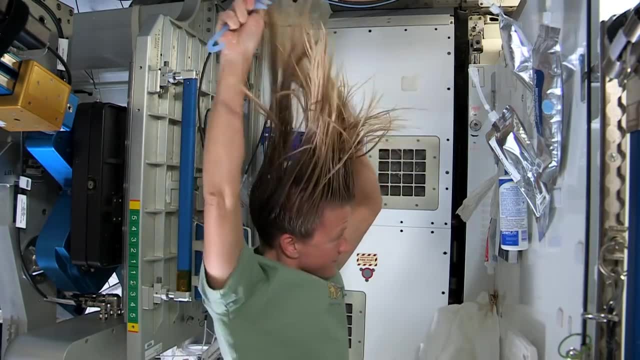 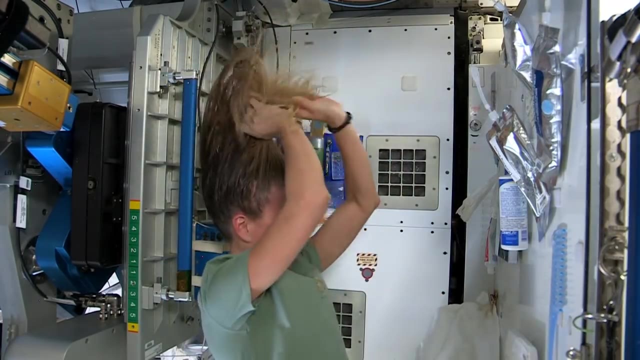 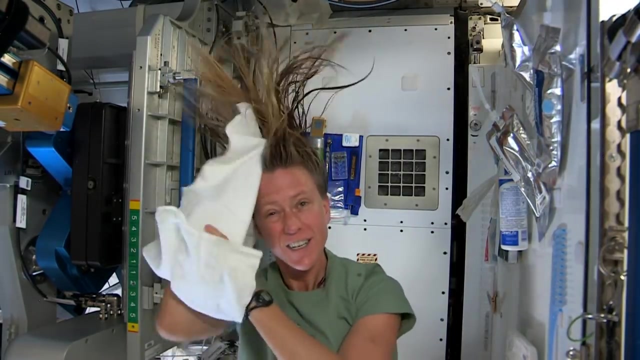 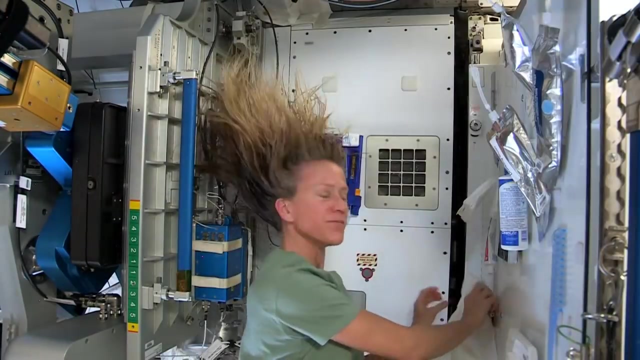 water with it. It actually feels kind of squeaky clean right now. Now I'll take the dry part of my towel. We used towels for quite a while here. Since we have limited supplies, we use them wisely There. I think that's pretty good, And now, as my hair dries, as the water evaporates. 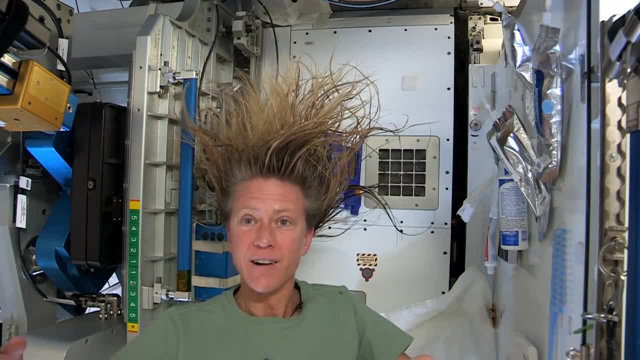 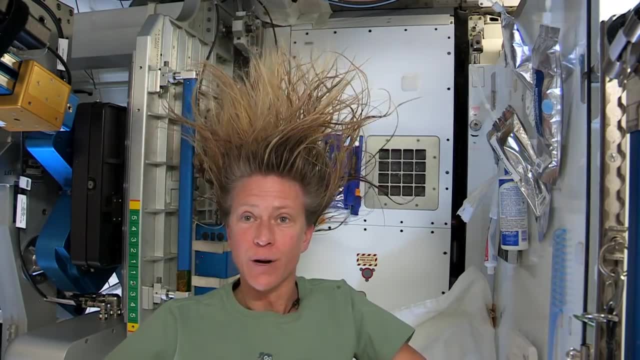 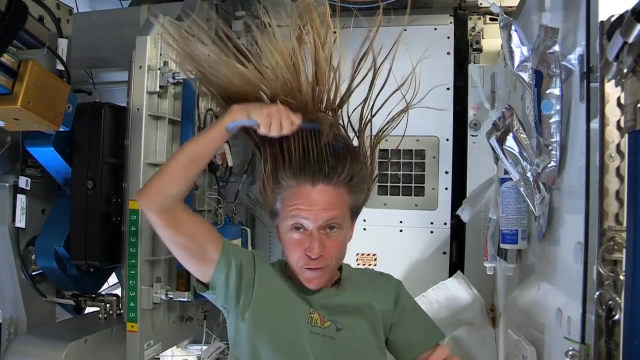 from my hair. it will become humidity in the air And then our air conditioning system will collect that into condensate and it won't be long, and our water processing system will turn that into drinking water. At the end I just do one final comb through to make sure there are no snarls and snags.